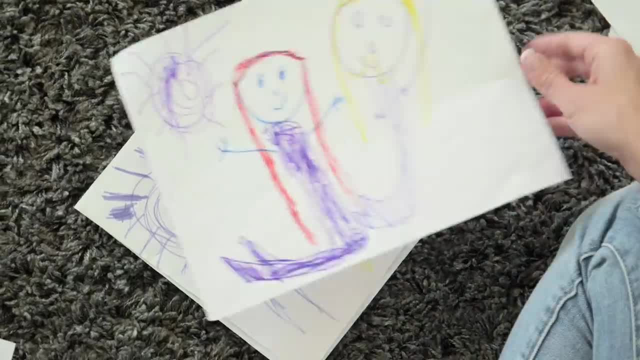 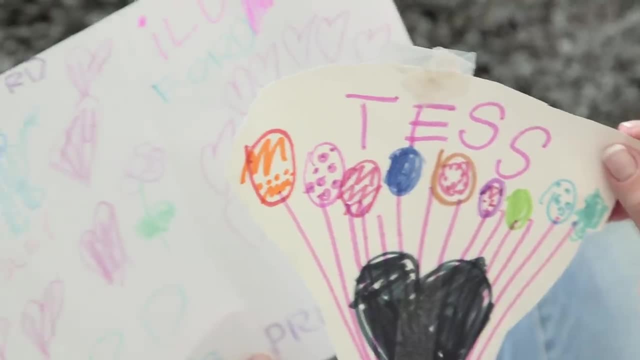 I have to keep one because she made a thousand of these. Help Presley loved mermaids and cats And she was obsessed with going to New York City. I think this is from the Home Alone 2 movie, Her pride in being a big sister. 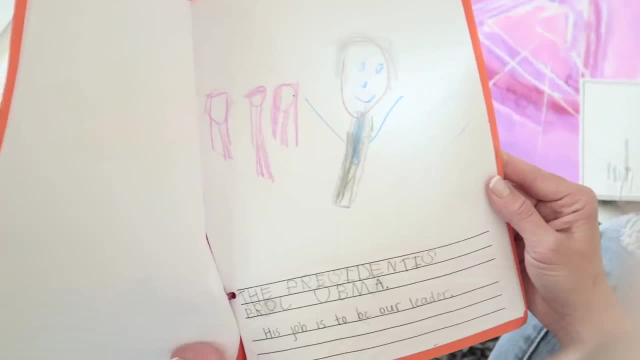 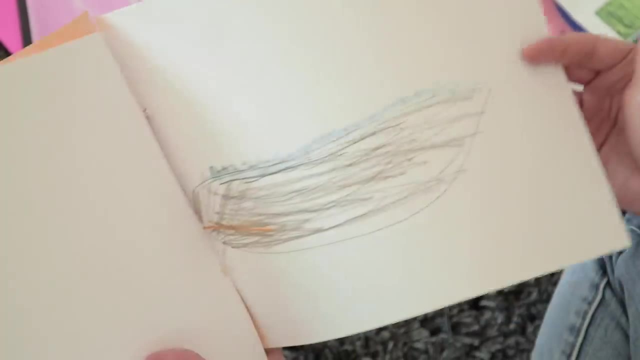 Look what your big sis made for you. Who was president? Good old B-Rock, Anything with a handprint. My weakness: I was less attached to caterpillars. What is that? Dots Any experiment with abstract art. At least they had the decency to laminate this. 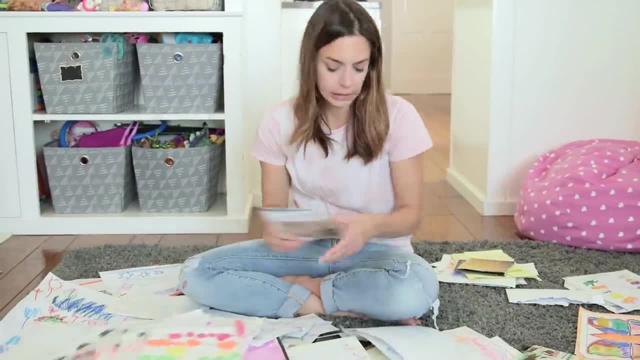 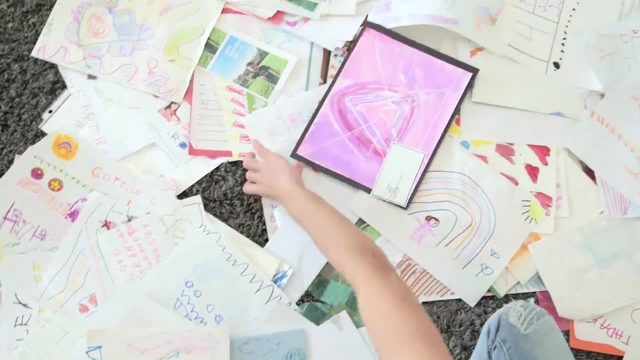 And I imagine this is going to get harder as they get older, with writing samples and report cards, But I'm going to keep trying to remind myself that it's better to enjoy a few special things than have so much clutter. you can't find anything. 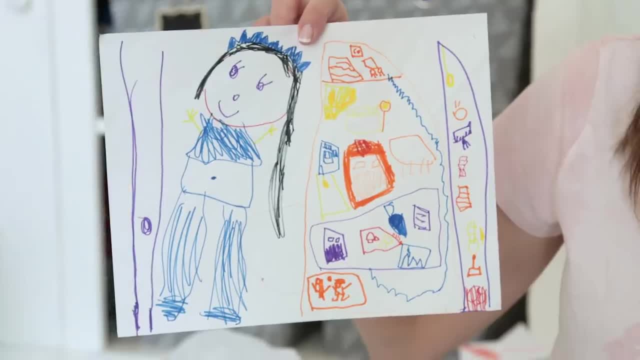 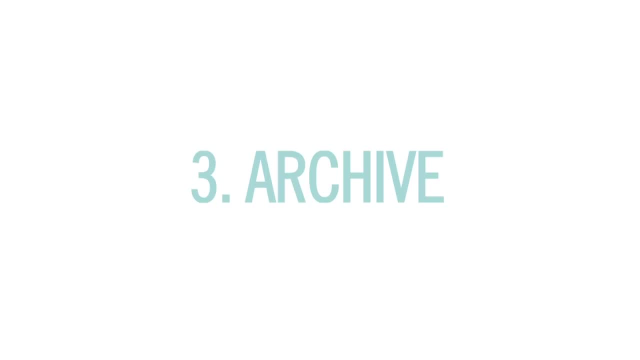 I don't even know what this is Like. is this a crop top? In less than 30 minutes I had about 25 pieces. I need these To put in the permanent archive. Each kid is going to get these waterproof plastic bins with hanging folders. 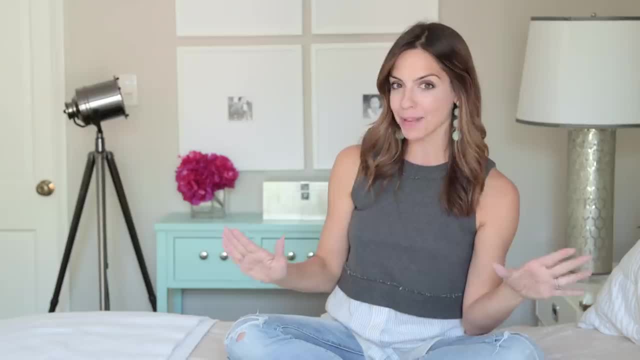 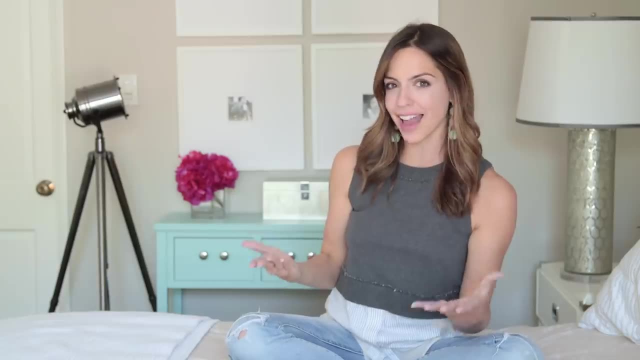 I'll link some options below And you guys, you can totally stop here, But if you want to go a little further, you can add in a picture, maybe of their first day of school. And then I actually wanted to write things down as my memory. 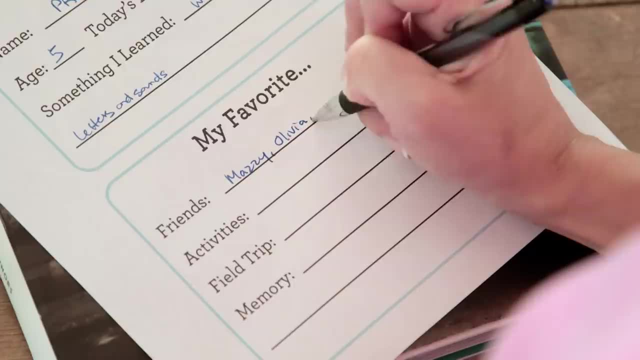 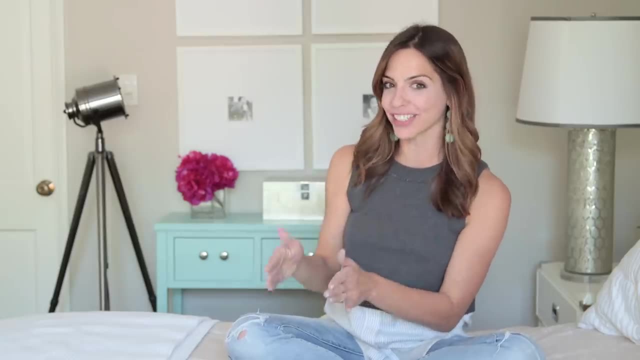 was jogging through the pile Things like their best friends, fun memories, the big things they learned throughout the year, And so I created this form. I'll also link below And I'm going to pre-stuff the folders because I feel like there's a better chance. 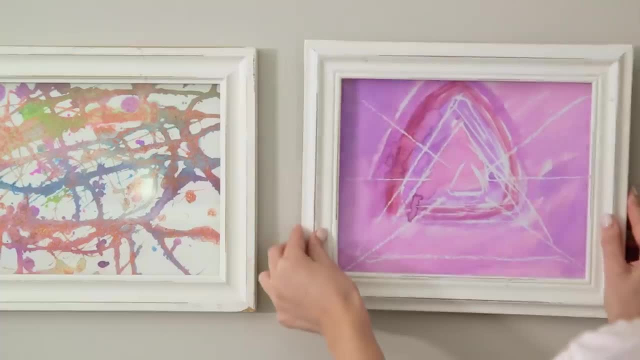 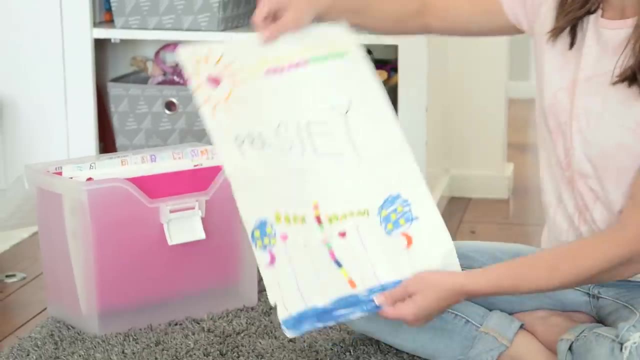 I'll actually keep doing this, Increasing the odds. I ended up framing some of the pretty colored paintings for the playroom, Giving a bunch to grandparents- Better late than never. And then for the bigger stuff that doesn't fit, you can actually roll it up into a mailing tube. 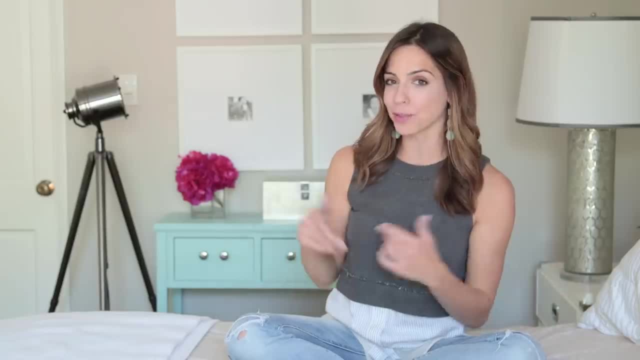 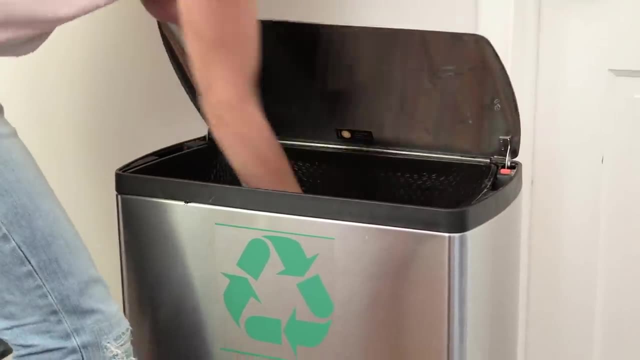 Or I just took a picture. I don't know if I'll ever upload it Or use one of those apps, But it made me feel a little less guilty when I had to say goodbye. I've got to really push it down, Cover it up with some stuff. 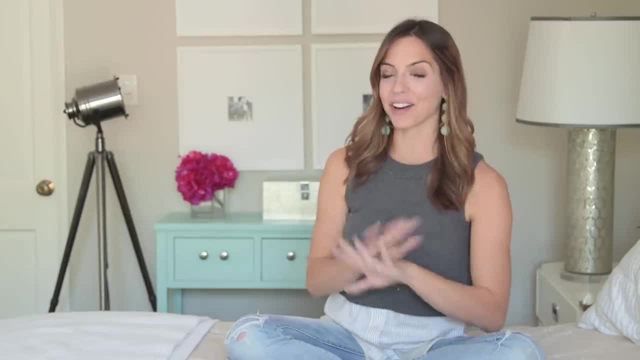 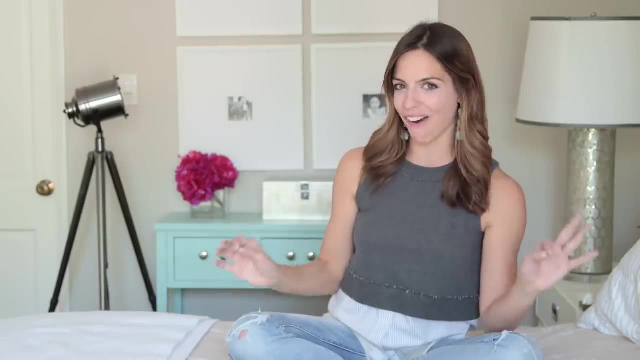 Speaking of, which definitely do this whole thing after the kids go to bed or when they're not home. Board Buddy- All right guys. So I hope this helped you develop a system for all that amazing artwork. I will see you next week. Bye.